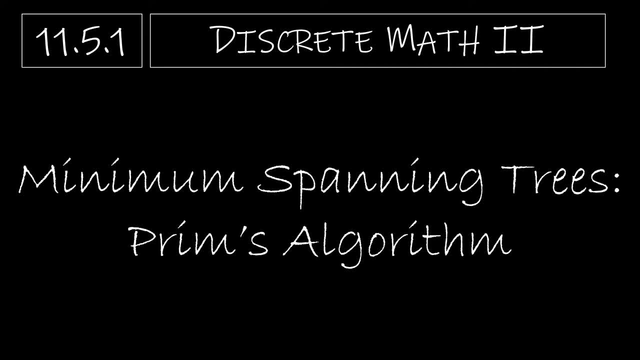 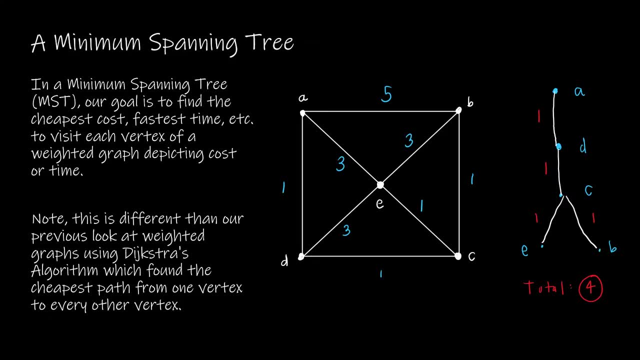 We're going to finish up our study in discrete math 2 combinatorics by looking at minimum spanning trees. We will begin with Prim's algorithm For a minimum spanning tree. obviously we're trying to create a spanning tree for a weighted graph and in this weighted graph, 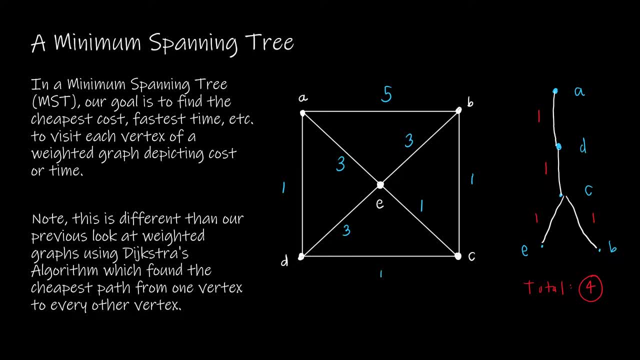 we are looking for the cheapest cost, fastest time or so forth, depending on what is being depicted on the graph. Now I do want to point out to you that this is different than our study of Dijkstra's algorithm. In Dijkstra's algorithm, we started with a vertex and found the cheapest. 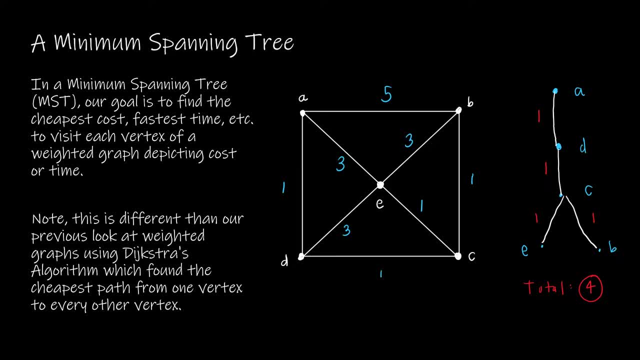 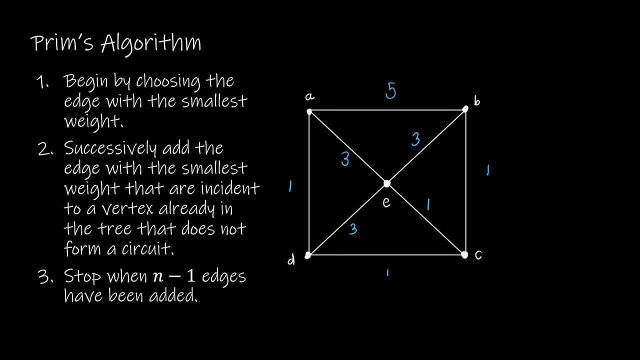 or shortest path to each other vertex. A minimum spanning tree obviously requires that we visit every single vertex. To begin Prim's algorithm, we are to start by choosing the edge with the smallest weight. Now in your textbook it says: choose the edge with the smallest weight In. 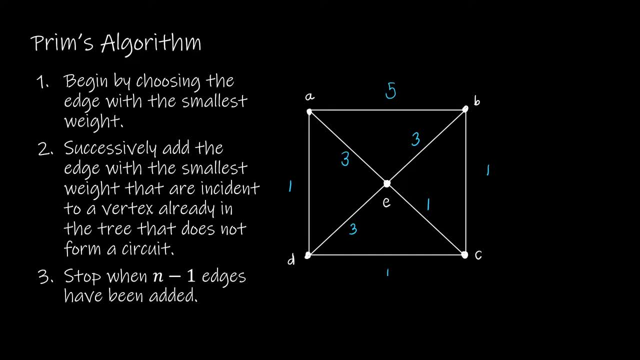 several other resources. it says: choose a starting point. just as we did for the spanning trees that we just looked at, We chose an arbitrary starting value, and that's what we're going to do here as well. So your textbook doesn't say to choose a specific vertex in which to begin. so you might see that written differently in. 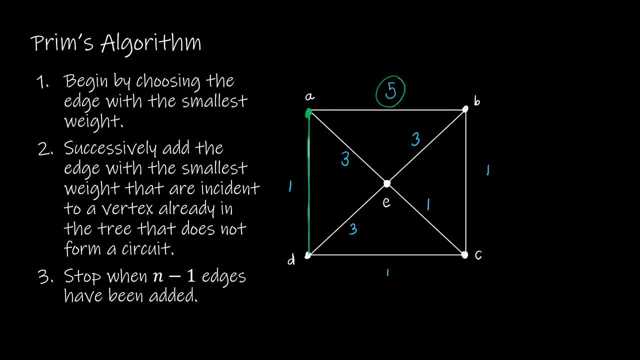 different ways. Now, from A I can go 5,, 3, or 1.. So I'm looking at those weights and this is our Dijkstra algorithm, so we're looking for the least of those weights. So, as you can see, I've sort of gotten ahead of myself and chosen. 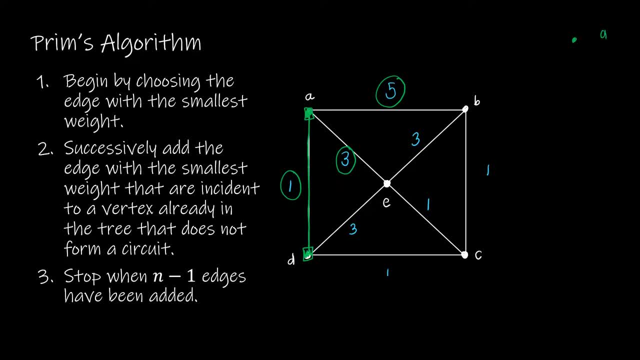 D. So as I'm drawing my minimum spanning tree, I'm starting at A and I'm going to D and I'm using a weight of 1.. Now Prim's algorithm says: from both A and D. so we're going from any vertex that we've already visited. 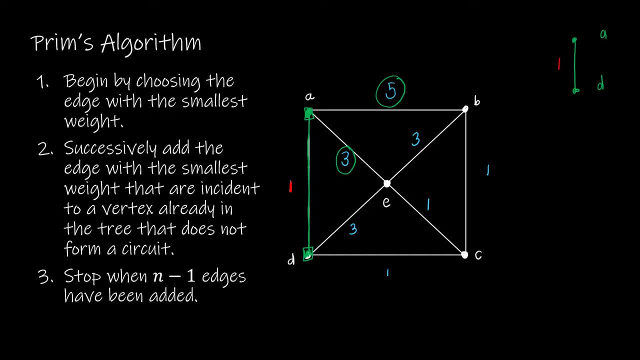 From both A and D. so we're going from any vertex that we've already visited. By the way, if you're in a去了 concept, you can already measure two vertices in each vertex, because even we've already visited. So from A I still have 5 and 3.. From D, I have a weight of 1 or a weight. 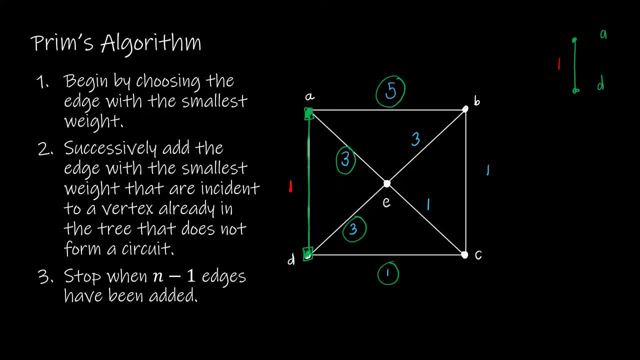 of 3.. So out of those three, I'm going to choose obviously a weight of 1.. So I'm going to choose to go to C, and C has a weight, DC has a weight of 1.. So now I'm still going to keep 5 and 3 and 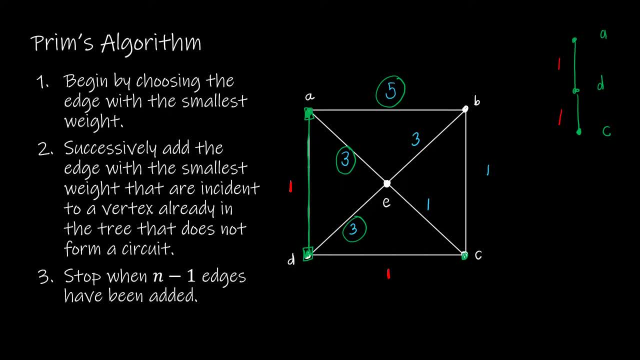 3 circled. But now, because I have visited C, I can also choose to go 1 to visit E or 1 to visit B. Now, when it comes to something like this, where you have more than one cheapest path, 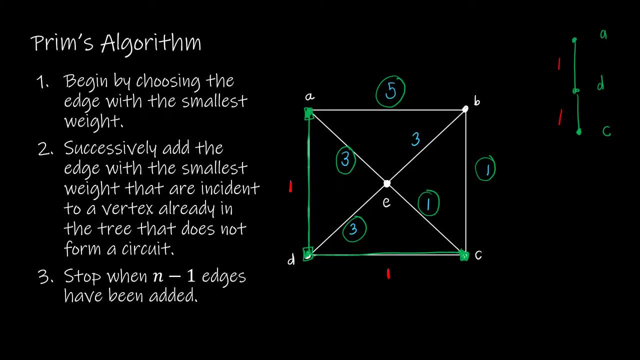 you get to choose whichever one you want, So I'm going to choose 1 and visit E. next, I'm going to go ahead and put the 1, since I already have the red color, So I'm going to choose to visit C. 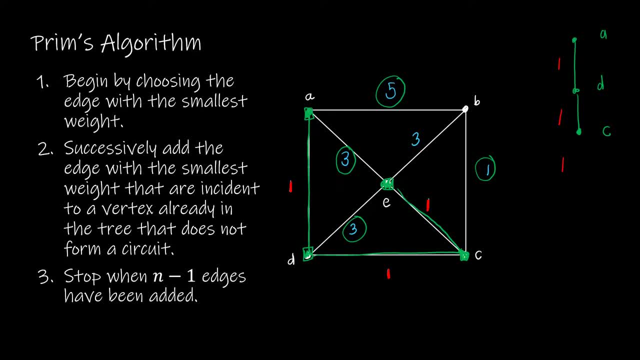 visit E, and that's a weight of one. Now, as you can see, I no longer need this three because I've already visited E, and I no longer need this three because I've already visited E. So, really, my only choices are one or three, because I can go from E to B, or five- Oops, I should keep this going over. 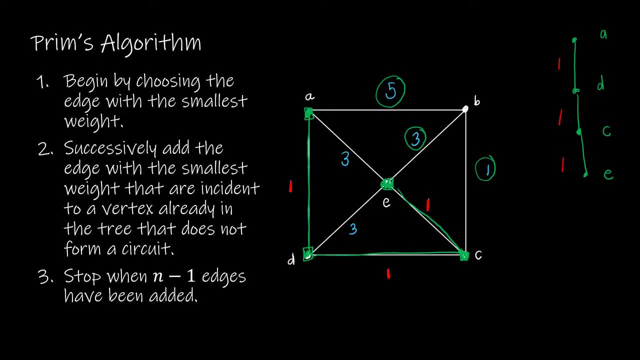 here. So this was E, And from E I can now go to B, And the shortest path to B is obviously the one, And so actually that's going to go from C. So I'm going to visit B, and that's also a weight of one. 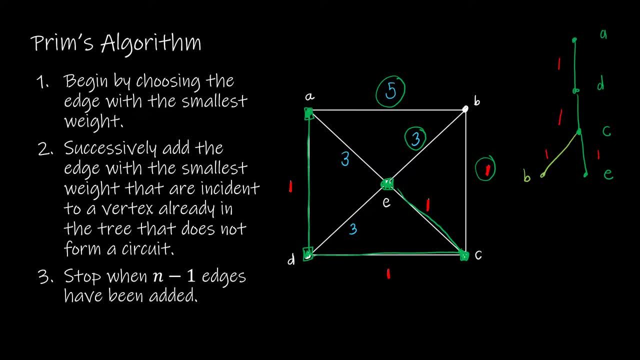 So this would be my minimum spanning tree. You can see that I have a lot of space here. So I'm going to go from E to B, So I'm going to visit B, and that's also a weight of one. So this would be my minimum spanning tree. 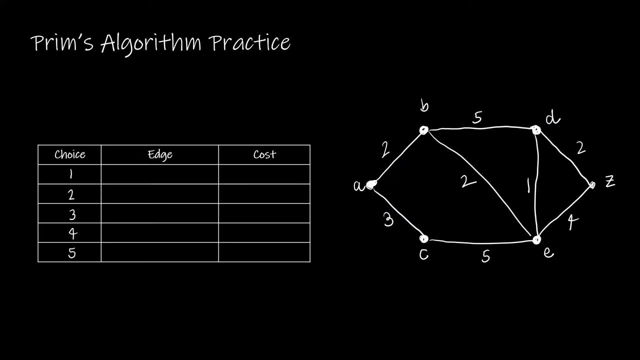 Using Prim's algorithm. we're going to go through this practice together and we're going to begin at A, So if it doesn't tell you where to begin, you would start obviously with DE, which is the cheapest weight. If it tells you to begin at a specific vertex A, then that's where you should. 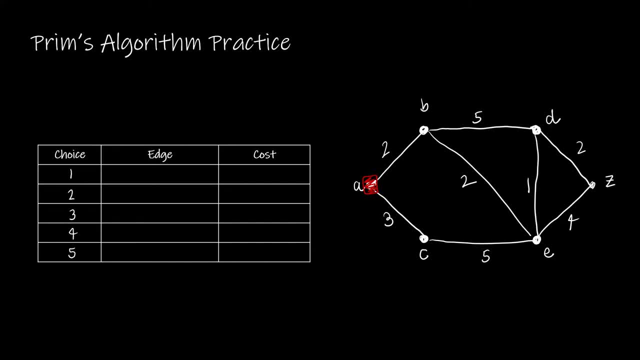 start. So if I have to start at A then I'm only looking at weights of edges incident to A. So from A I can choose 2, or I can choose 3.. So the cheapest of those obviously is from A to B. 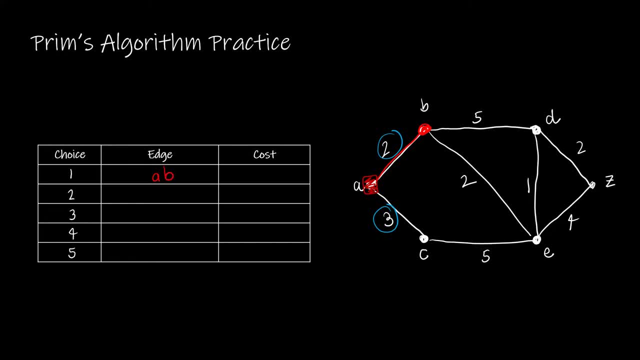 So I'm going to choose edge AB with a cost of 2.. Now, from here, I'm going to think about any of the other vertices that I can now get to, based on A and B both being visited. So I can choose to use 2 coming off of B. 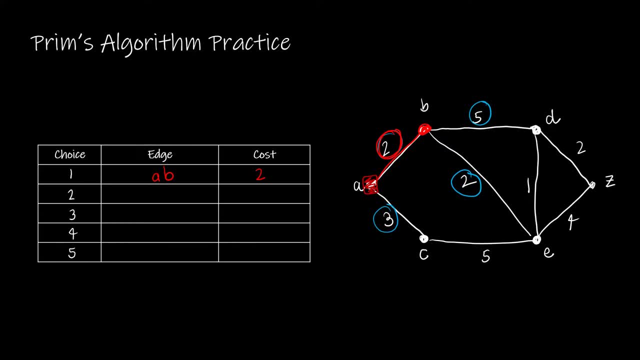 Or 5 coming off of D, And again I'm looking for the least cost. So the least cost of those is 2.. So I'm going to add BE And that's a cost of 2.. Now, from E I can get to C by a cost of 5. I can get to D by a cost of 1.. 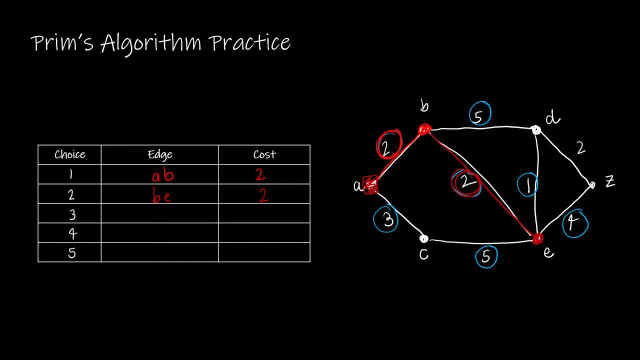 Or I can get to E, Sorry Z with a cost of 4.. So, again, I've still got all of the values circled that I can use, And that's just for me to be able to see more clearly which one I should choose. So I'm going to choose. 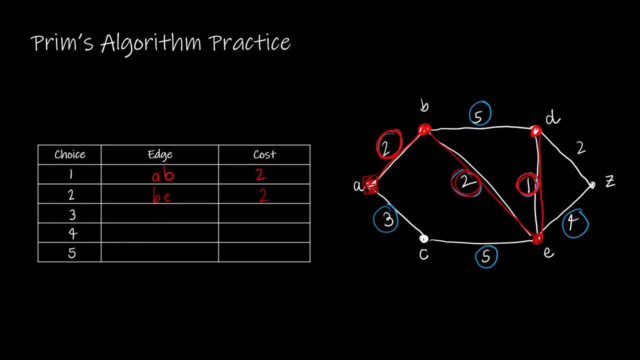 a weight of 1 because that is the cheapest. So I'm going to add edge ED, And that is a cost of 1.. Now can I get rid of any of the circles that I have so far? I can get rid of them, So I'm going to add a weight of 1.. And that is a cost of 1.. 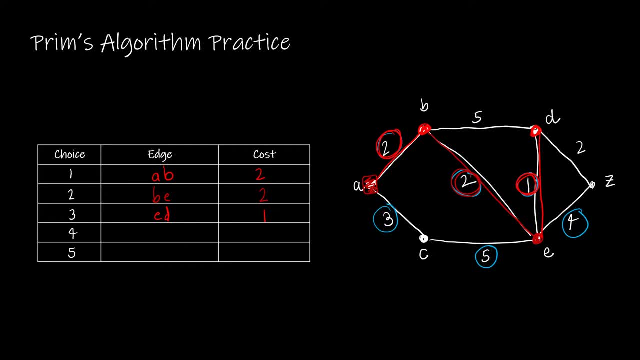 I can get rid of 5 because B and D are both already visited. So what I have left is that I can add 2, because that is the last weight, And if you want to somehow mark off the 5 to show that it can't, 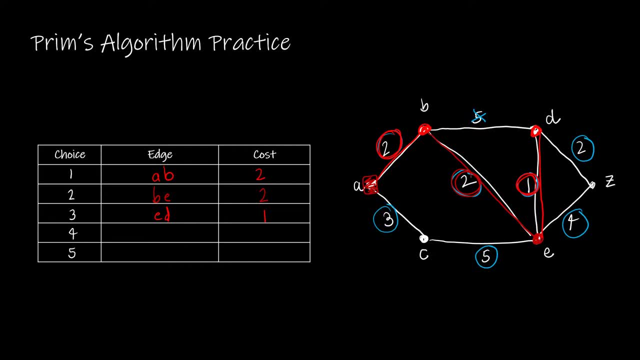 be used. you can certainly do that as well. So from here I'm going to choose. out of all of the values that I've circled, 2 is the least. So I'm going to go from D to Z. Obviously, I'm not going. 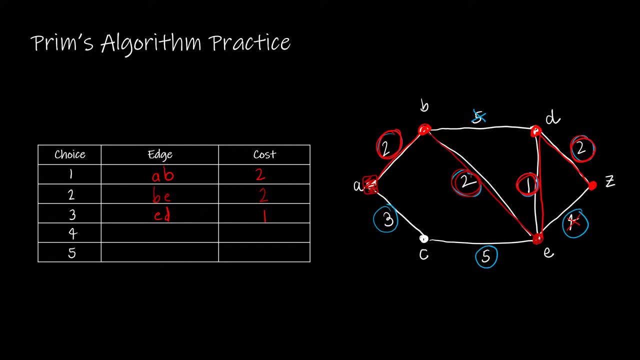 to use 4 anymore. So I'm going to go from D to Z And I'm going to go from D to Z And I'm going to use 4 because I've already visited both E and Z, And so really all I'm looking at is 3 and 5.. So 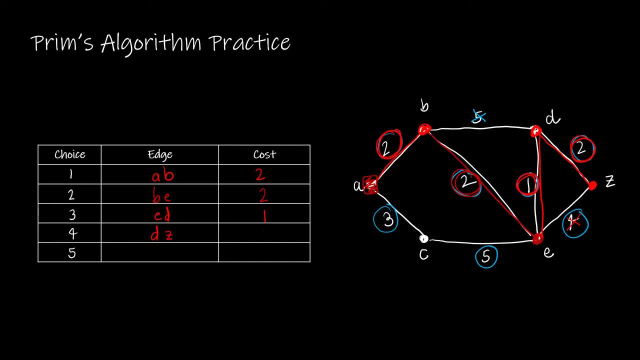 let me write down that I did DZ with a cost of 2.. And then again between 3 and 5,, 3 is the cheapest choice, So I'm going to go from A to C with a cost of 3.. So my total cost is 2 plus 2. 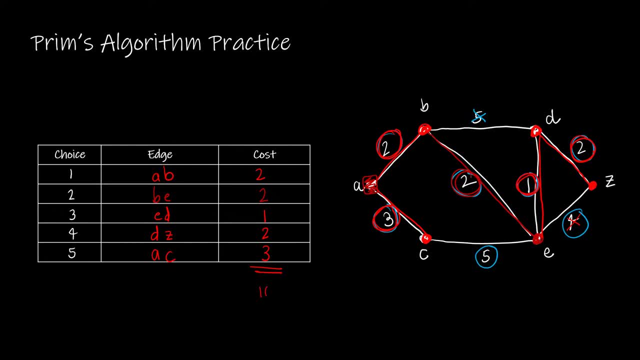 plus 1, plus 2 plus 3, which is 10.. And I should also write or draw my minimum spanning tree. So I chose to begin at A. Now A branched off into both B and C, And AB had a weight of 2 and AC had a weight of 3.. From B: 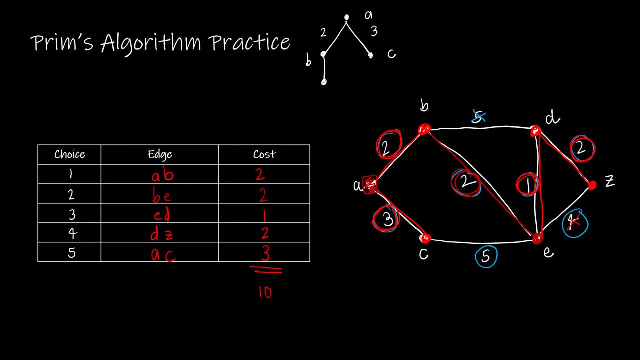 I branched off into just E with a weight of 2.. From E to D to Z. So from E to D was 1. And from D to Z was 2.. Probably a good idea to use a different color for those weights. But that's 5,, 7,, 8,, 9,, 10.. So you can see that I have a total minimum. 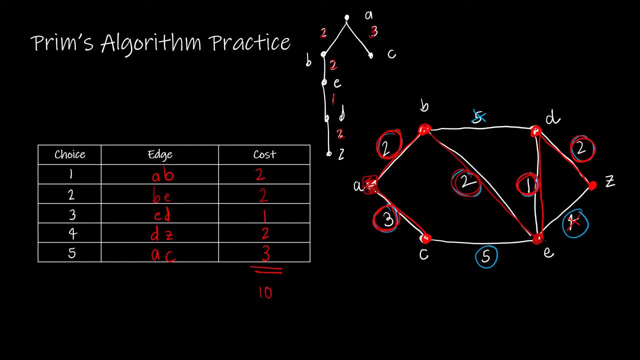 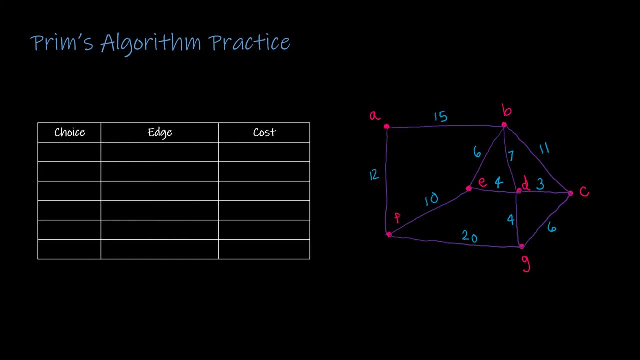 spanning tree cost of 10.. And that is what the minimum spanning tree looks like. Try this last question on your own. When you are ready, press play to see how you did. Before I get started on this one, I do want to point out to you that creating a table isn't. 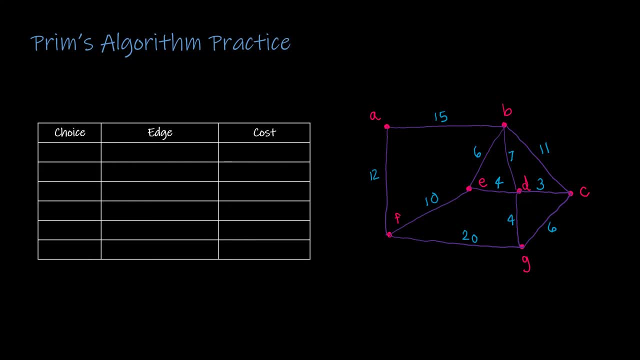 necessary to use the algorithm. I'm asking you, as your instructor, to create the table so that I can keep track of what you did at each point. It makes it easier for me to make sure that you understand how to use the algorithm correctly. So again, how many choices will I need to make? Remember? 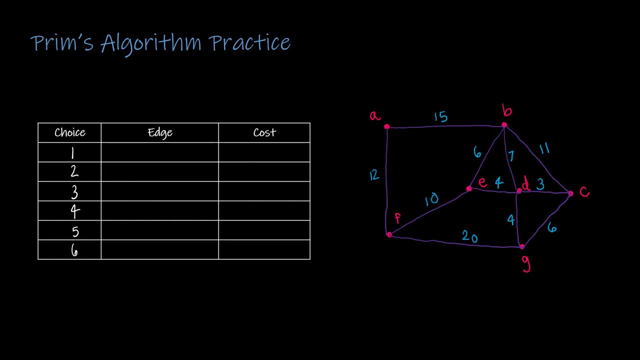 we are going to make N. That's how we'll know that we've made it to the N, And N, of course, is the number of vertices. So in this case there were 7 vertices, so I'm going to make 6 choices. Now again, if I'm asked. 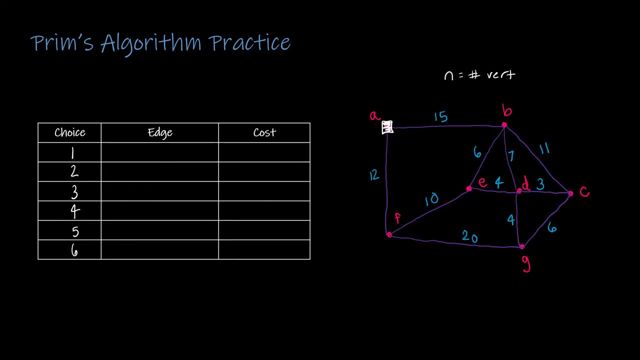 to begin at A. it's going to look a little bit different than if I'm asked to just use Prim's algorithm. So for this particular case we are going to choose just the cheapest. So I'm not going to ask you to begin at A Now. hopefully you're going to be able to do that, But if you're, 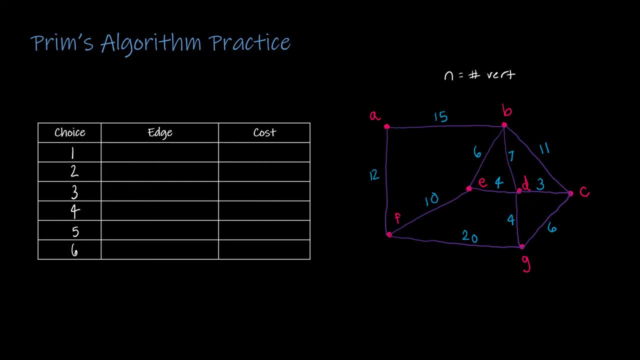 going to choose to begin at A, you will end up with the exact same solution whether you chose to begin at A or not. So, looking at all of the values on my graph, I'm going to start with DC with a weight of 3.. Now, from DC, I can choose 11.- 11.. I can choose 6.. I can choose 4.. I can choose 4., Or I can. 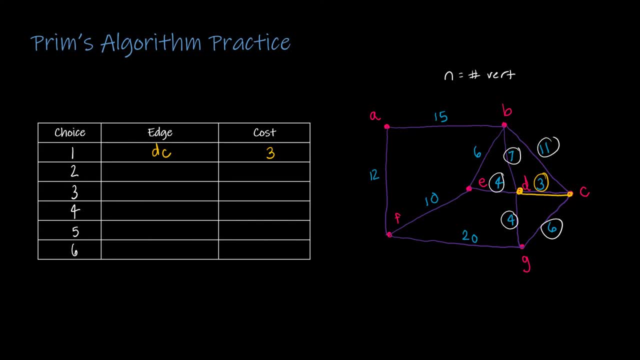 choose 7.. So which one do I want to choose? Well, obviously one of the 4s And I'm going to choose DG. So DG has now been added with a weight of 4. And I'm going to think about anything coming off. 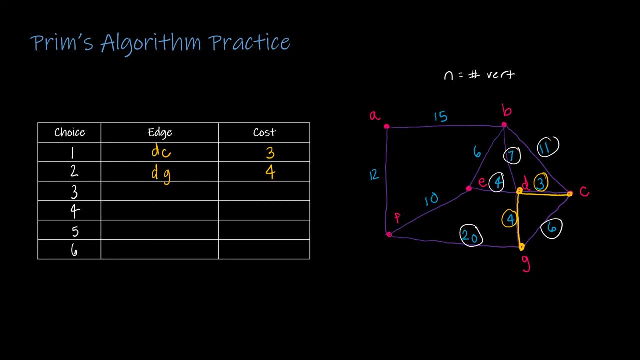 of that. So I'm going to add 20 as a potential And I'm going to get rid of the 6. So you can erase it off, You can erase whatever. So now looking at what I have: 20,, 4,, 7, and 11.. 4 is the. 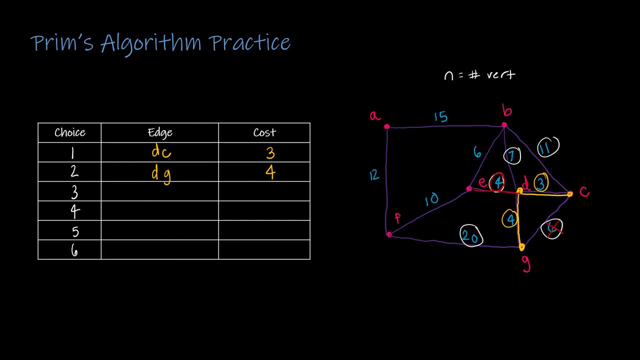 cheapest, So I'm going to choose 4.. So that is ED with a cost of 4.. So 4 has been chosen, And I'm now going to consider also a 6 and a 10.. So of the values that I have, I'm going to choose 4. And I'm 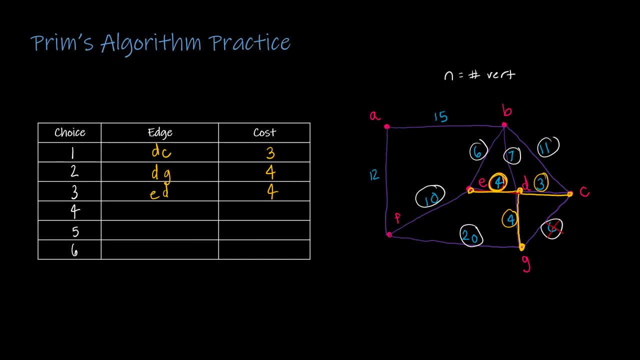 going to choose 6. And that's EB. So EB with a cost of 6.. Now I can get rid of the 11 because I've now already visited B and C, And I can get rid of the 7 because, again, I've already visited all of. 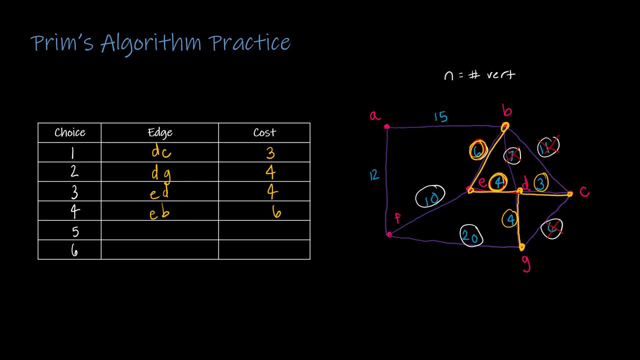 the values that are adjacent to that edge or incident to that edge. Other vertices I can now or other paths I can now take. I can use the 15. I can use the 10. Or I can use the 20.. So the